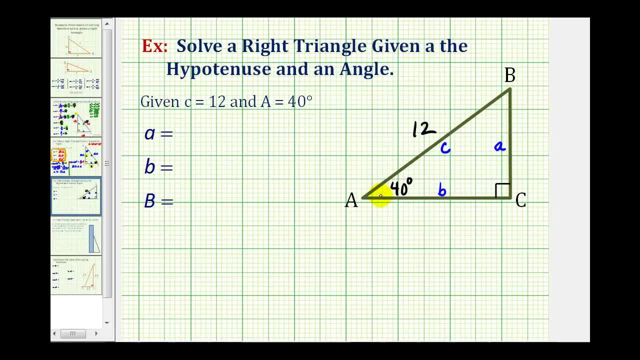 that the two acute angles must be complementary or have a sum of 90, which means the measure of angle B must be equal to 90 degrees minus 40 degrees. so the measure of angle B is 50 degrees. Now we'll have to find the length of side A. 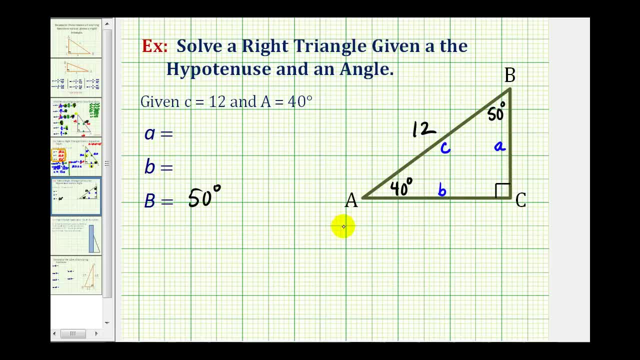 and the length of side B. To do this we'll have to use a trig equation. So let's first decide which angle we're gonna use. Let's say we're gonna use angle A and we wanna find the length of side A. 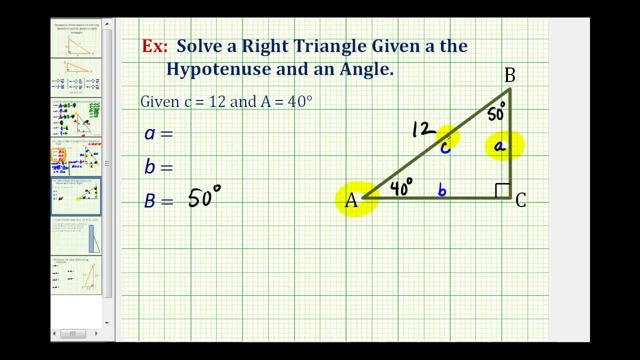 Well, we know we have to use the length of side C because we know the value of C and we can only have one unknown in our trig equation. Notice that A is the opposite side of angle A and C is the hypotenuse, and since the sine function involves the opposite side and hypotenuse, 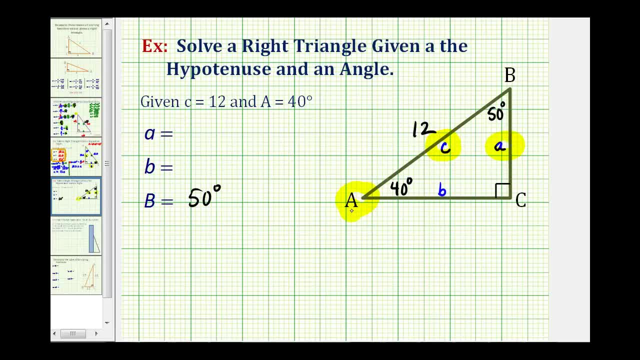 of a right triangle. we know we have to use the sine function in our trig equation. So our trig equation is going to be: the sine of forty degrees must be equal to the ratio of the opposite side to the hypotenuse, or in this case a divided by twelve. And now we need to solve this equation for a. 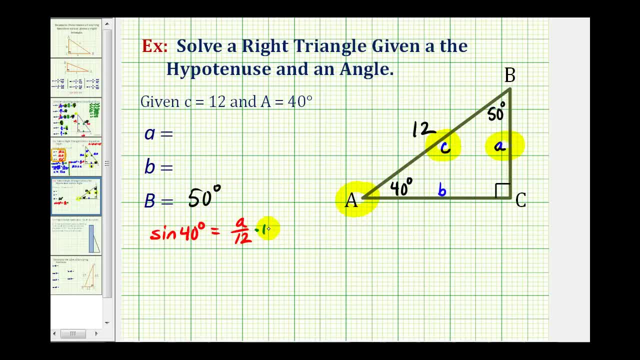 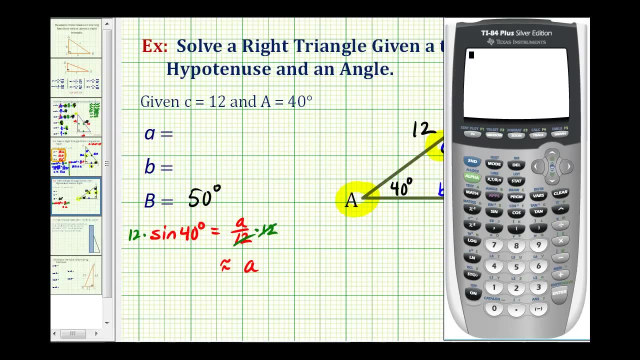 so we'll multiply both sides by twelve, So the right side simplifies to a. So a is equal to this product here, which we'll approximate using the calculator, One of the most important things we need to do is to make sure our calculator is in degree mode, So I'm going to press the mode key. 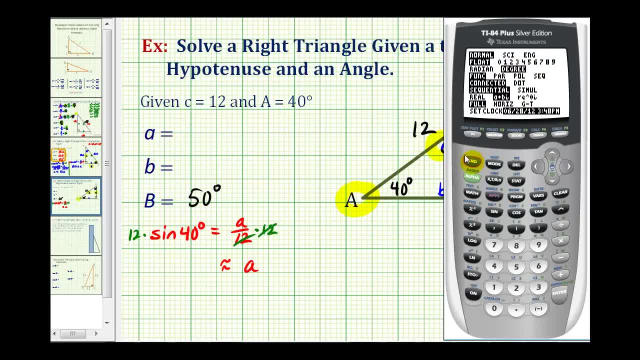 Notice, degree is highlighted. so we are in degree mode. So now, from the home screen, we'll approximate this product Twelve times sine forty degrees To the nearest tenth. this would be approximately seven point seven units the length of side A. 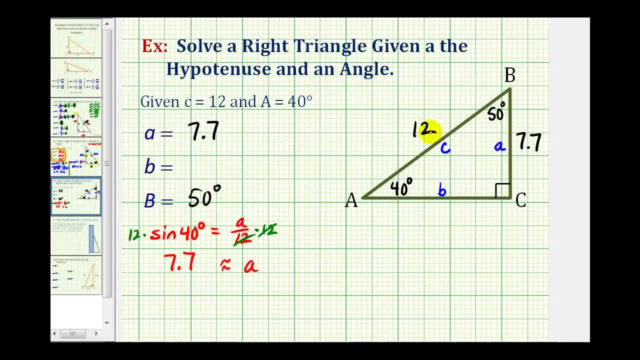 Now we're left to determine the length of side B, because now we have the lengths of two sides of the right triangle. we could use the Pythagorean Theorem, but I'm going to go ahead and use another trig equation. Let's go ahead and use.